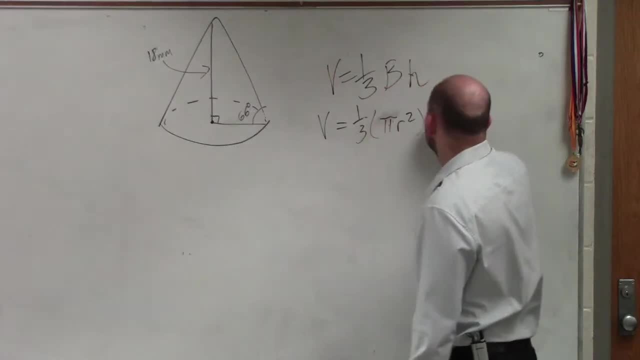 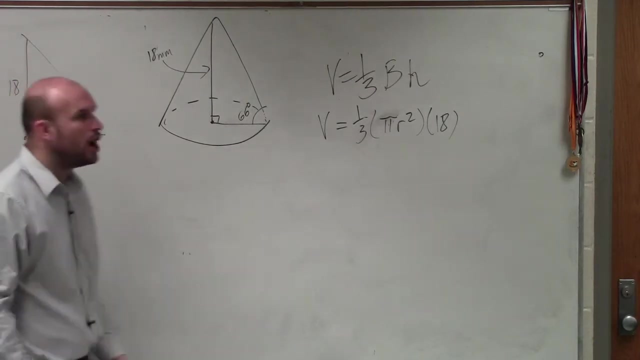 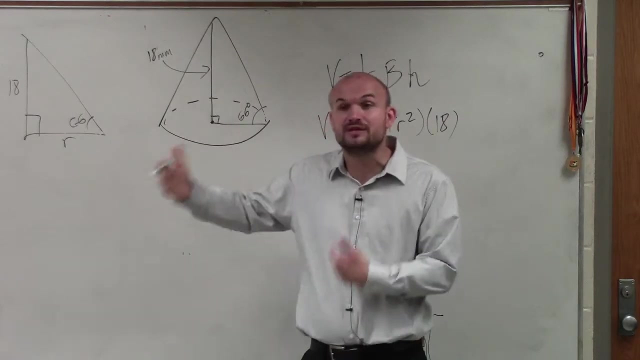 tell us. remember, the height is directly from the base to the top, which is 18.. So the problem is, we need to figure out what r is, Imani, because they don't tell us what r is. They do give us, however, a triangle And they say: that's 18 and that's 66. We need to figure out r. So to do that, we have to use our special right triangles. That's 66 degrees, not 60 degrees. If that was a 30-60-90, you could use your special right triangle relationships, But since it's not 60 degrees, 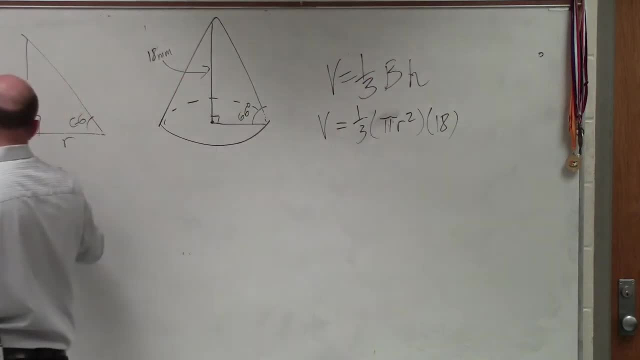 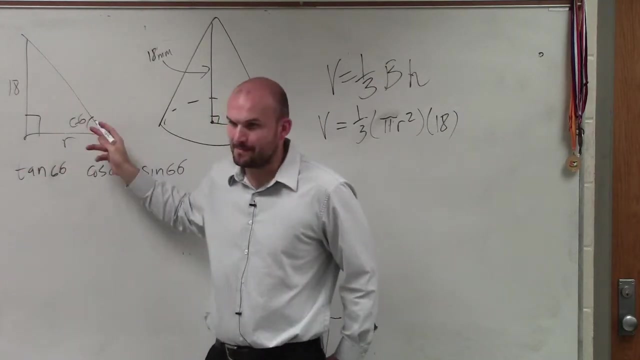 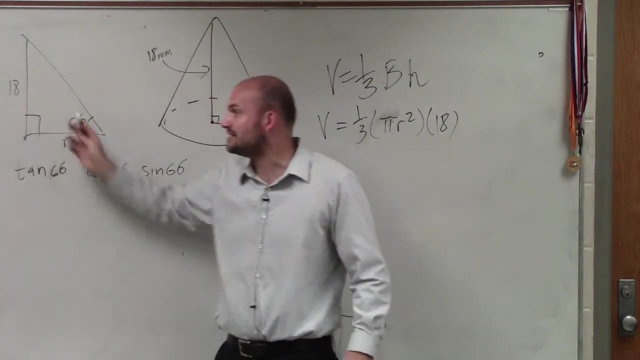 it's not a special right triangle. therefore, I have to use either tangent of 66 degrees, cosine of 66 degrees or sine of 66 degrees. Now, since we need to now look at what we're given, well, remember, r is your adjacent side and that's your hypotenuse. So therefore, since we don't have a hypotenuse, 18 is our opposite side. So the only function that deals with opposite and adjacent is tangent. So I need to do tangent of 66 degrees. 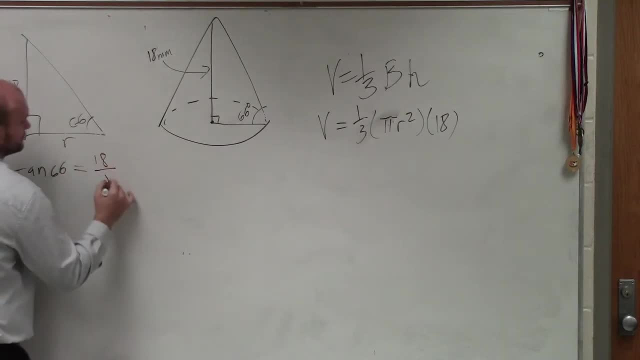 is equal to opposite over adjacent. Now I need to solve for r. So to get r off the bottom, I multiply by r on both sides. Therefore now I'm left with r times the tangent of 66 degrees equals 18.. To solve for r: stay seated, please. Tangent of 66 degrees. 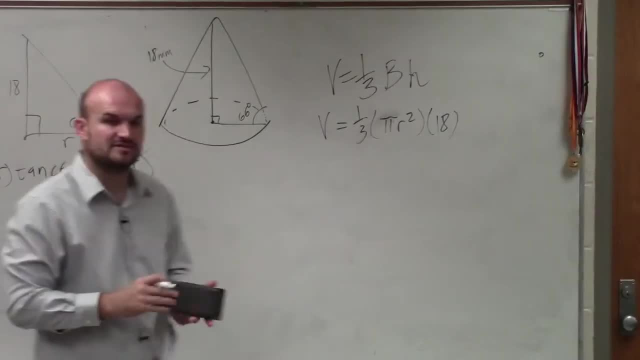 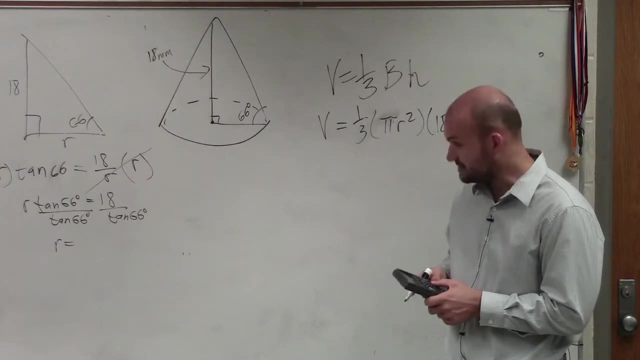 So, therefore, r equals 18 divided by tangent of 66.. So therefore, I now need to take my calculator, which I'm not done yet. 18 divided by the tangent of 66 degrees, That's going to leave me with r. 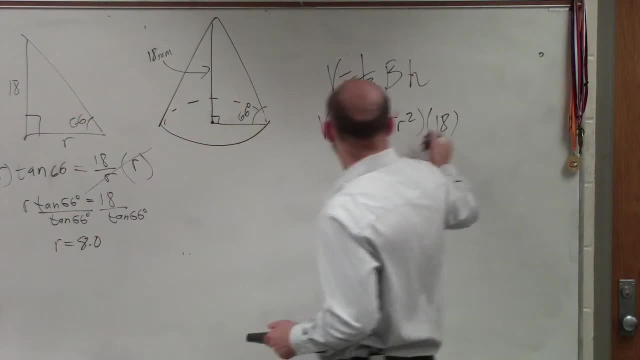 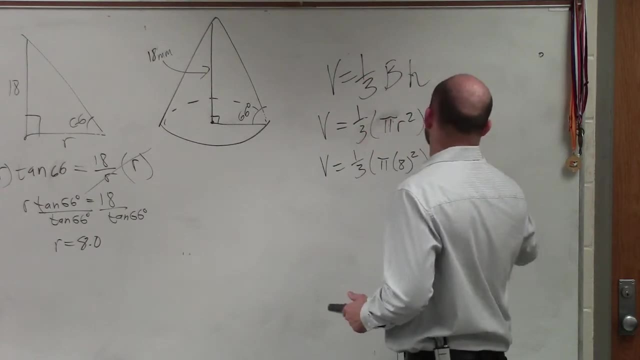 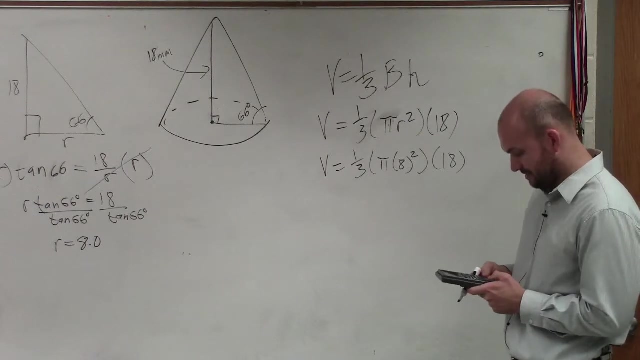 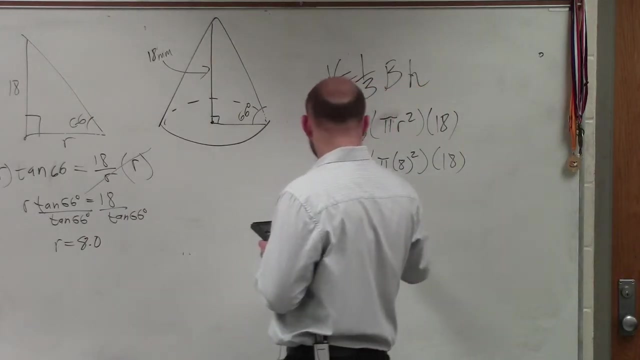 equals 8.0. as I round to the 10th, I now plug in that. So therefore I just take 1 divided by 3 times pi times 8, squared is 64 times 18.. And the volume of this is going to be 1,206.4.. Remember, this is millimeters. 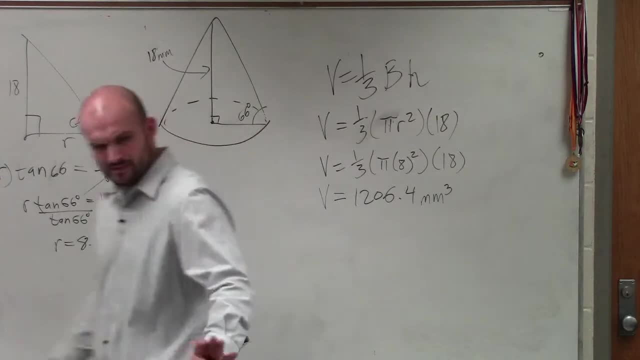 And since we're talking about volume, that middle- excuse me, well, the middle meters- is going to be Tyler. Tyler, excuse me, is going to be cubed.